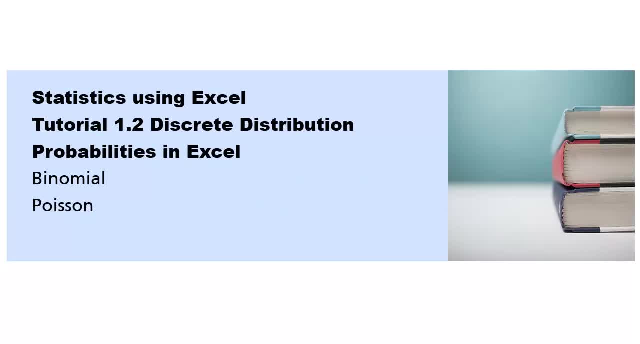 Welcome to this video on statistics using Excel. In this second tutorial, I am going to demonstrate to you how we can compute the probabilities for discrete statistical distributions using Microsoft Excel, And we are going to do it both for binomial as well as Poisson distribution. 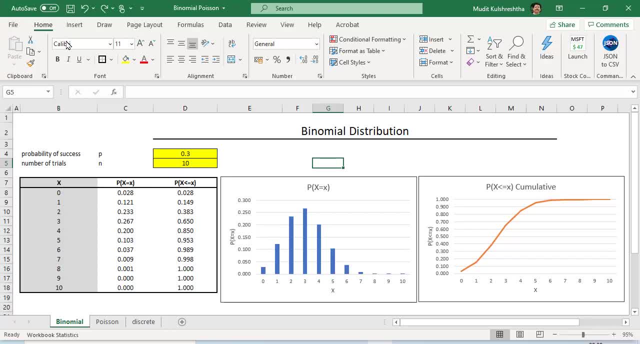 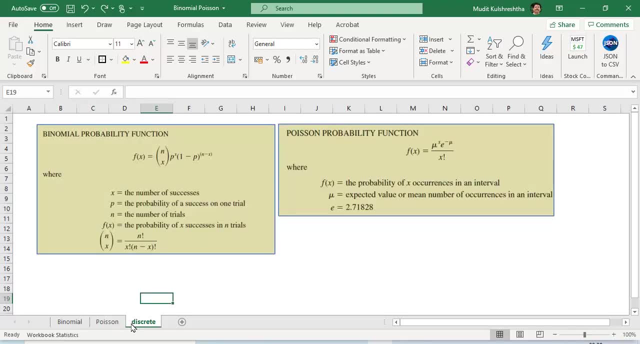 This is the Excel sheet that we want to replicate, one for binomial and the other one for Poisson. As you are already aware that discrete statistical distributions are nothing but a statistical formula to compute specific probabilities for a specific value of a random variable x. But we don't want to use these formulas directly. we want to compute these in Excel. 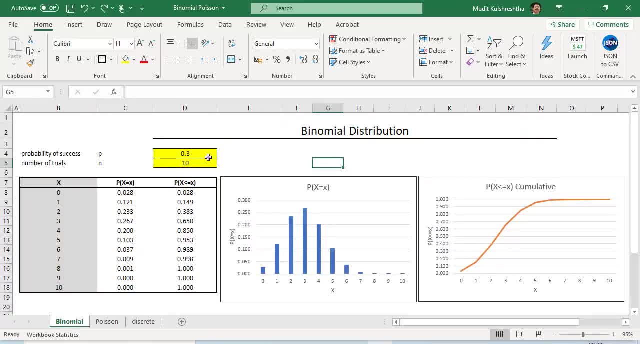 So let's get started. So this is the sheet that we want to replicate. On this sheet, we are replicating the binomial probabilities. Binomial distribution actually requires only two parameters: the probability of success and the number of trials. So, and what we want? 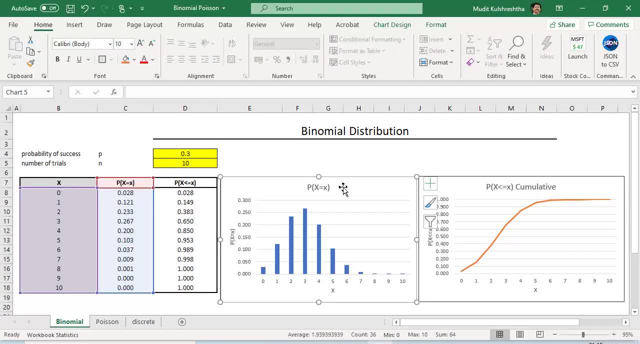 is this one table and we want these. So we have two graphs, basically one for the normal probabilities when random variable takes a specific value, and the other one for cumulative. So now let's replicate the sheet. What we also want is that, if we change these parameters, the numbers and the graph should 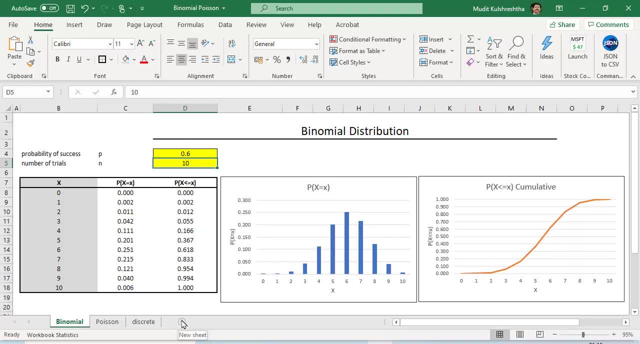 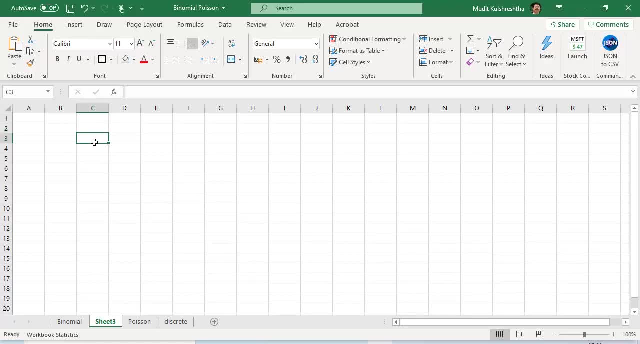 automatically change like this. So let's get started. Let's add a new sheet. Now let's start typing, for I require two parameters: One is the probability of success, denoted by small P, and then number of trials, which is n- Let's say this is 0.3, the original value and number. 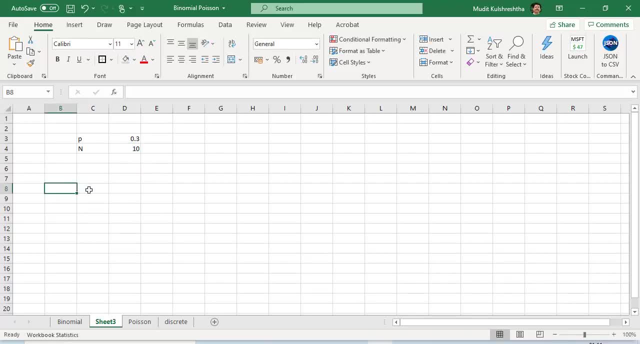 of trials are equal to 10.. So the random variable now we know is x and it can take the value of 0,, 1,, 2, 3.. Let's replicate very quickly up till 10.. And here I want the probability. 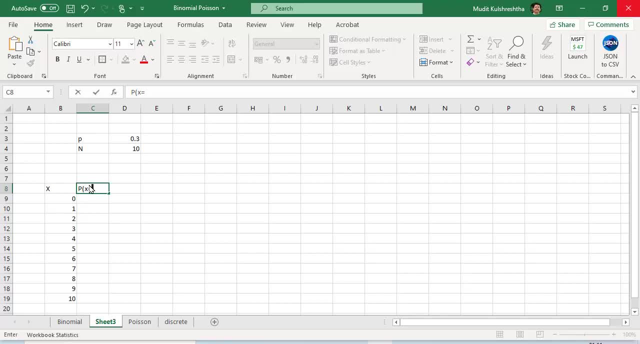 where x random variable can take on, can take on a specific value of x. And here we want cumulative whereby the random variable x, denoted by a per case letter, x can is less than or equal to x. So this will give us cumulative. Now 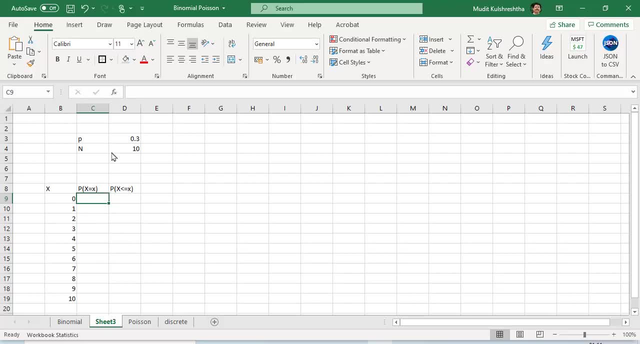 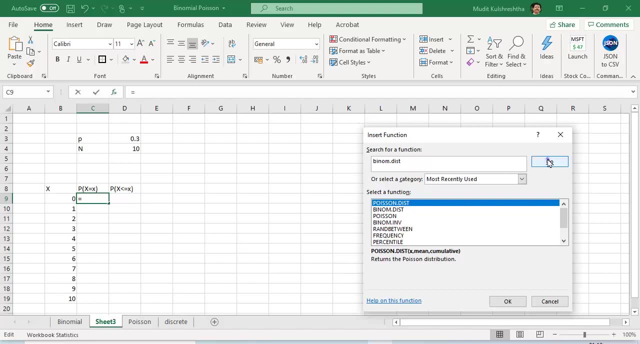 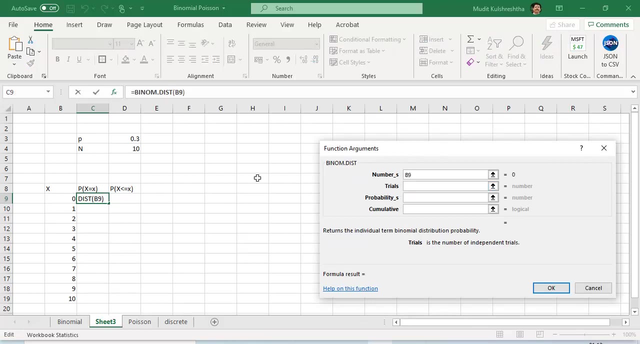 we are ready to use a formula. The formula to be used is binom dot dist. So I go to fx, I search for binom dot dist formula. just press go. this is the formula that i have. it says numbers and then the trials, which is this: 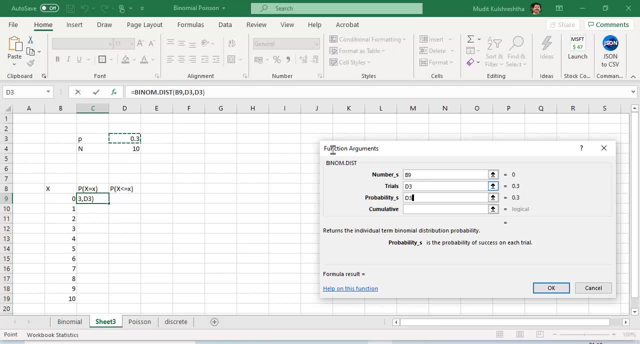 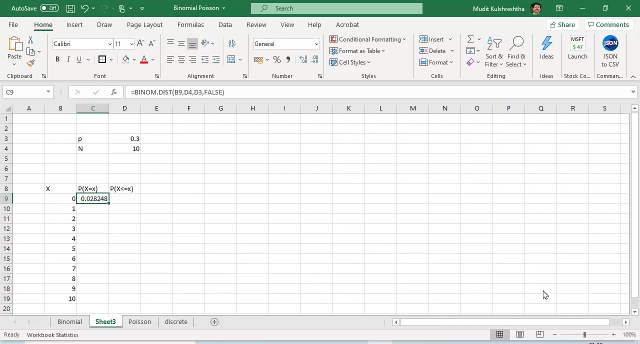 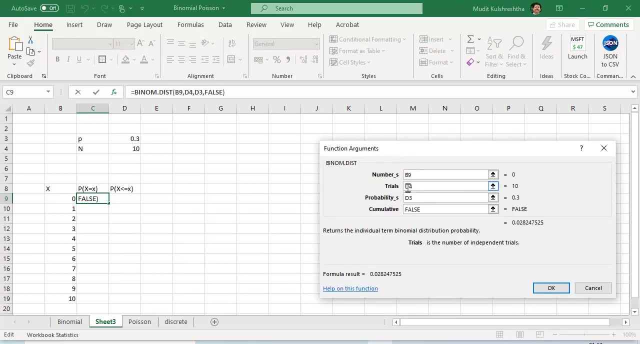 value and the probability is this. sorry, the number of trials is this and cumulative. we want false because we are looking when the random variable takes a specific value. so and we get our probabilities. now to make make a drag down, I need to supply the dollar sign. yeah, so which means which will go. 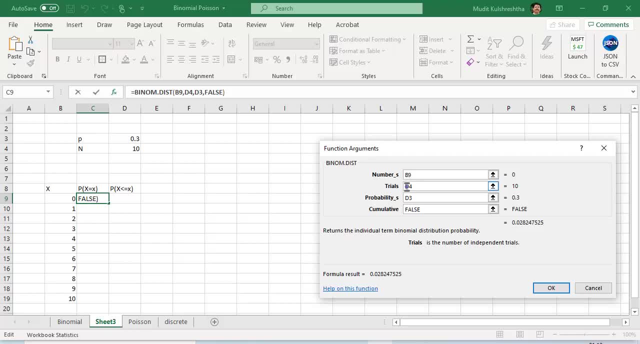 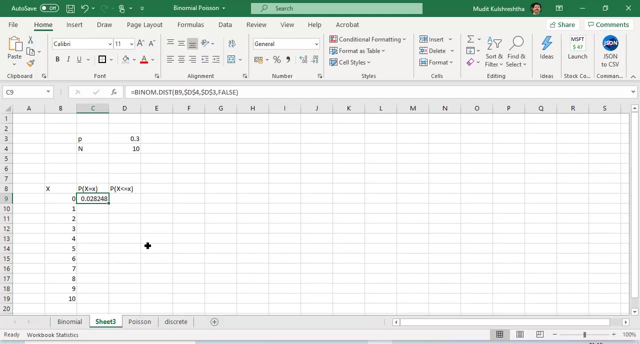 if we quickly tightly dollar, you can also use the f for button on your Excel and that's it. and now we can drag this. now all that you need to do is this: this x plus I esemp. Turn On by helping saya n. your an FanX, and this is also one way to solve this. it's an exactly similar to tort already in. 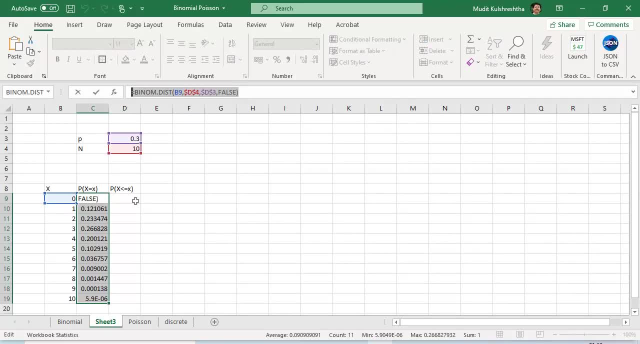 this. let's dump a eines, and i will. yet there is another important step to I combined all the values do for cumulative is that. copy this formula, because it uses the same cell, put it in the adjacent and, instead of false, make it true and this gives us the cumulative probabilities. 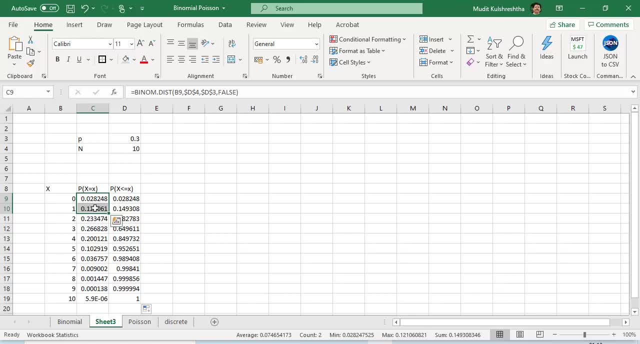 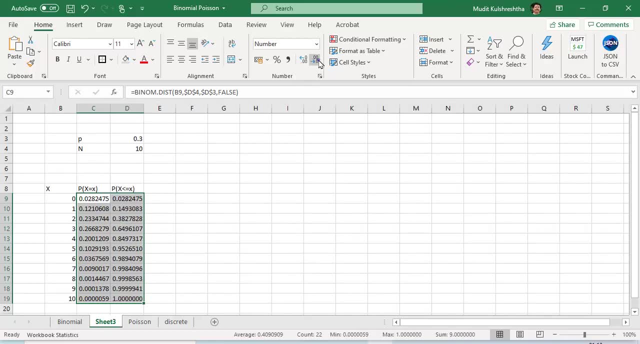 as you can see the. so now what we can do is quickly change the decimals to reflect the uniformity up to three decimal points. this is looking good. now we need to generate the chart. so the first chart that we want to generate is based on these two columns. just select them. 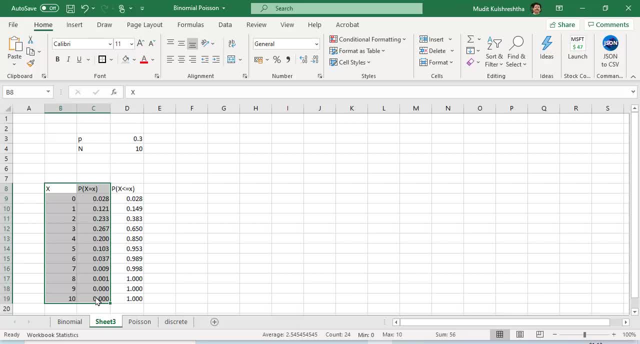 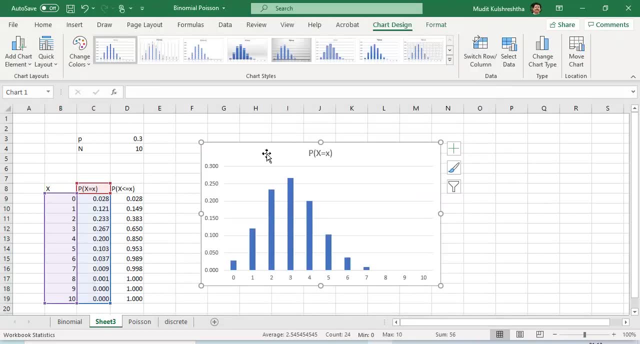 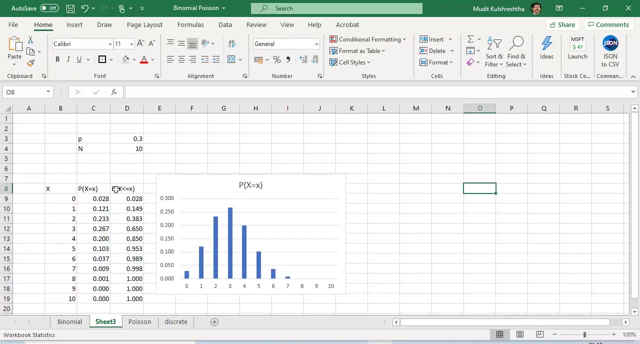 including the header. access is pretty intelligent in figuring out the right sort of chart. go to insert recommended charts and this is a chart that we are looking for. just type it here and just make it a little bit smaller. the another chart that we are looking for is: 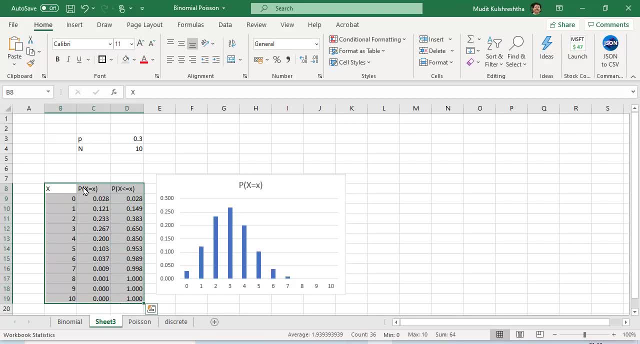 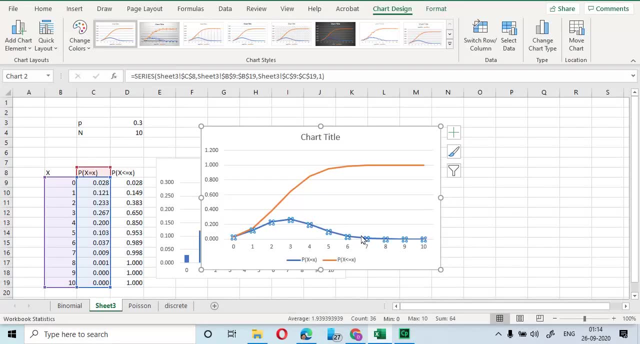 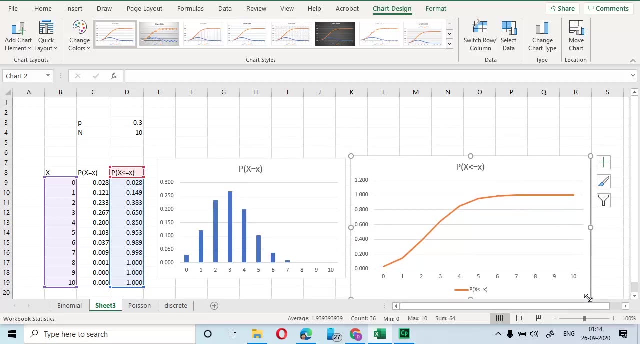 the cumulative chart. so choose all the three. go to insert. go to recommended charts, choose this one, press ok, just delete the second row and now we get the cumulative chart as well. so just drag it here, resize it now. let me very quickly reformat this sheet so that it: 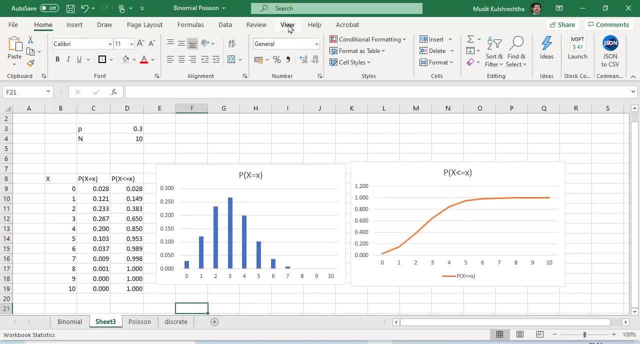 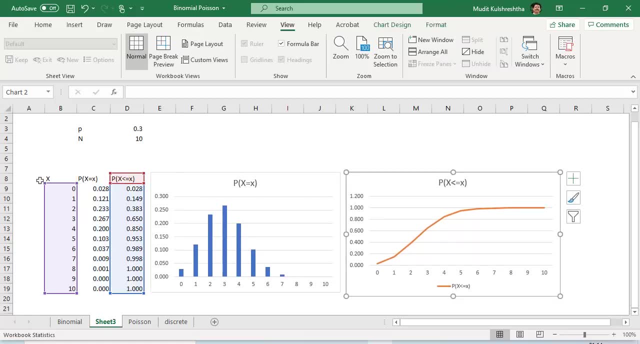 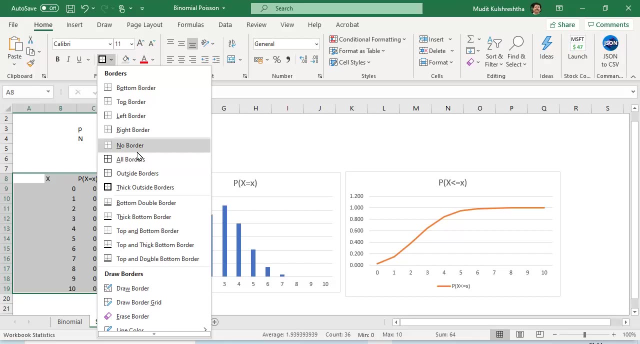 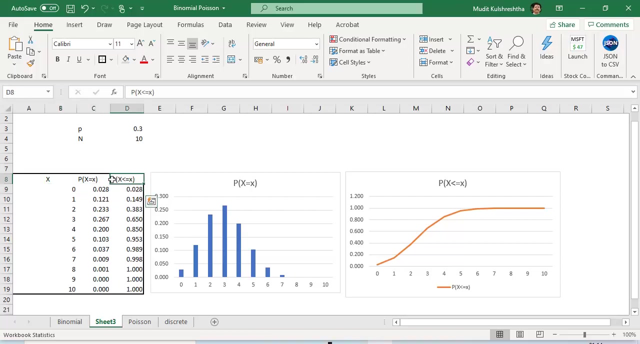 looks more readable. what I am going to do is go to view, make the grid lines disappear. that makes it neater. format this table a little bit to reflect. so I am going to provide it a grid based, not a grid based structure. let me provide it a border. I think this will do, so let's make 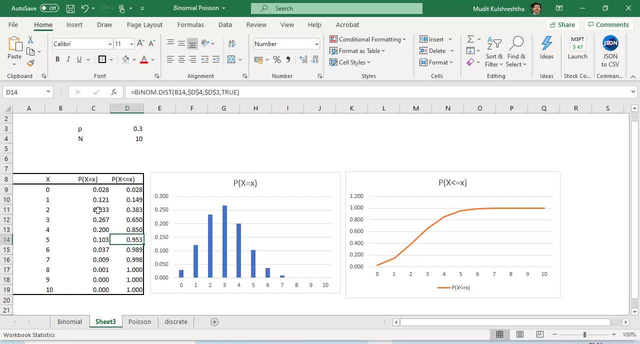 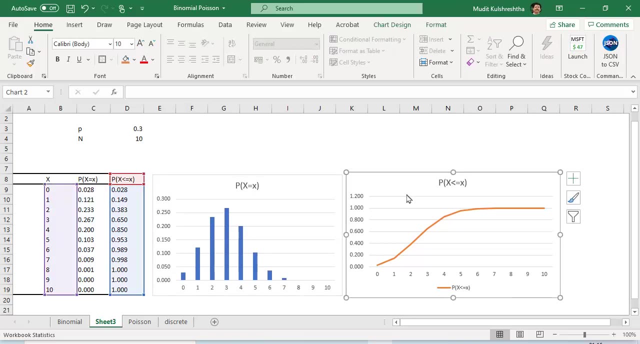 this left aligned, make these middle aligned, or make these also left aligned. I think that will look better. so now the table is there. what you can do is, in this particular graph, you know that cumulative probabilities will never exceed one, so I want to make this axis equal to one. I double click on it: make this. 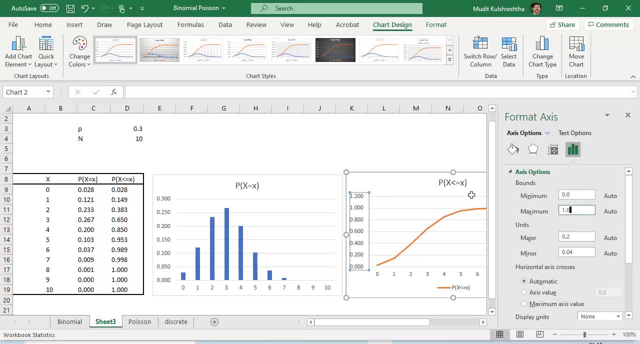 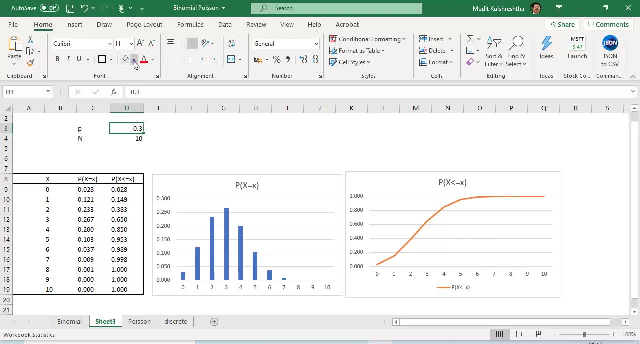 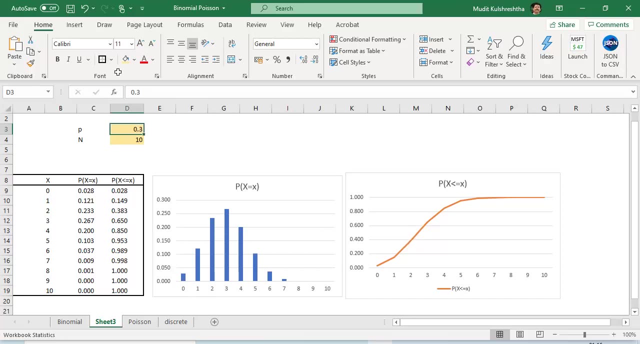 maximum value equal to one point zero. and now this is looking better, so you may want to color this a little bit and provide it a border, so that you know these are the parameters and also the differentiation between these two curves, so don't change this. and this is. 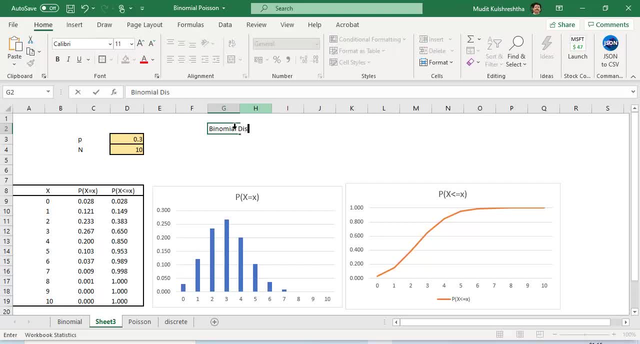 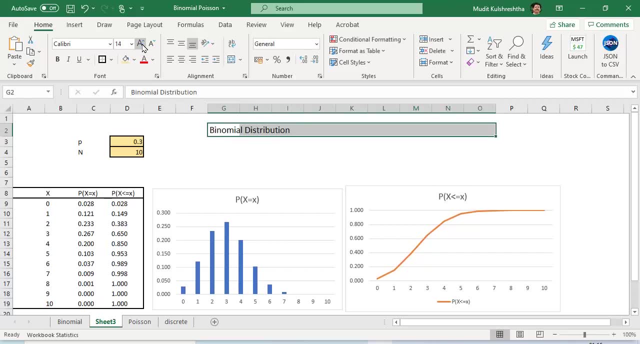 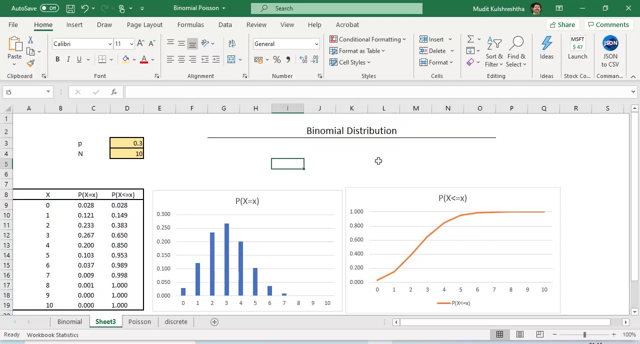 my binomial distribution. just provide a header, make this a little larger, center it and just draw a bottom border, and this is the sheet that we're looking for. so from this you immediately get the probabilities, and if you change this to 0.6.5, you may be able to get the probabilities. 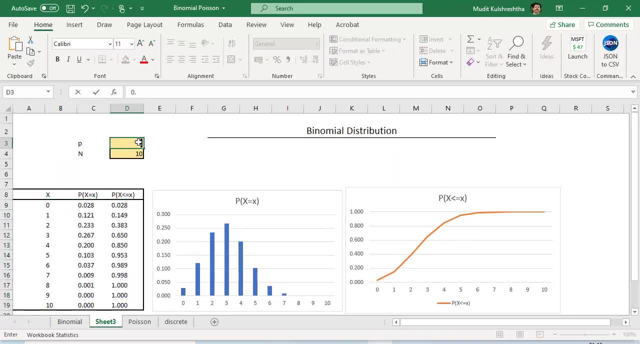 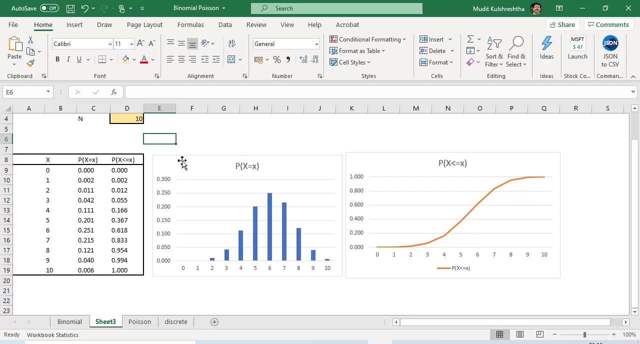 more easily. all the probabilities in the graph will also change. so with that, now we are ready to replicate this sheet for Poisson distribution also. so now let's quickly do the sheet on the Poisson distribution. the best way to do it quickly is to replicate this same sheet. 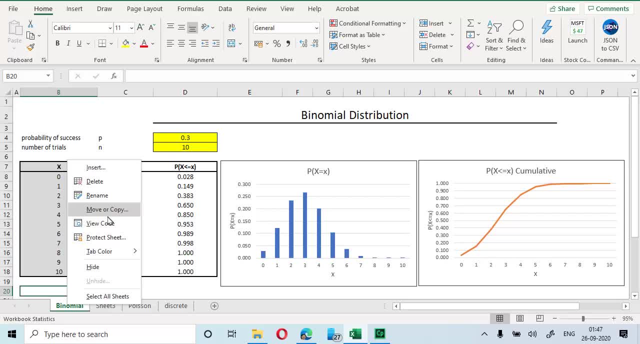 making it changes for the things that are required in Poisson distribution. so I am going to copy the sheet. I am just going to create a sheet. let's name it P2, and now I am ready. so, basically, I am going to first change the header and we require only one parameter. 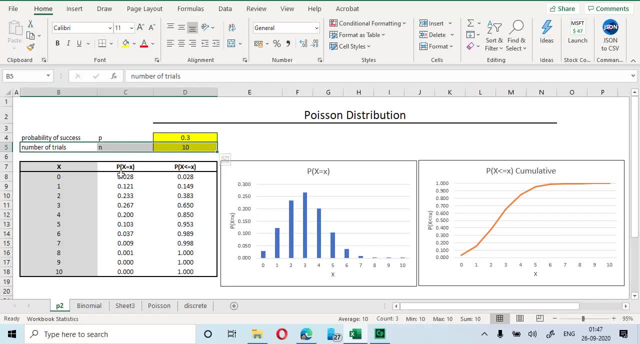 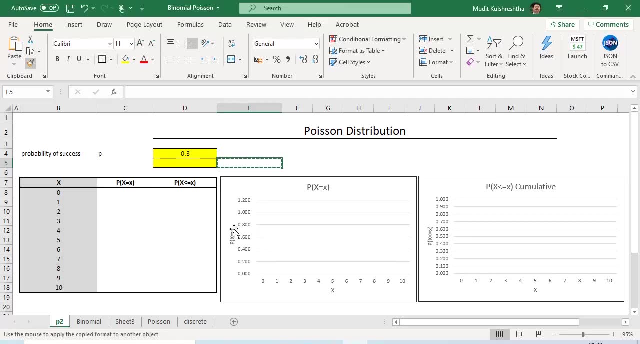 so this will not be required. but let me first delete these values in the table. so now we have a template, we don't require this parameter, so this can be deleted. now, the only parameter that Poisson distribution requires is basically arrival rate. mean so, Poisson distribution, one major example that we associated with. 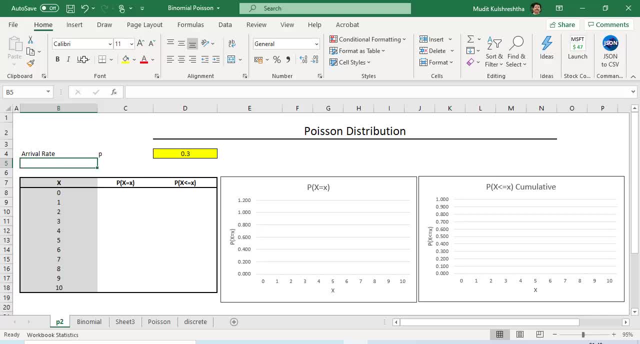 is with arrival of customers on a service counter or arrival of calls in a call center agent or the number of cars arriving at the toll station in unit of time. so let's say there are three cars arriving on the toll booth and now we can compute the probabilities. 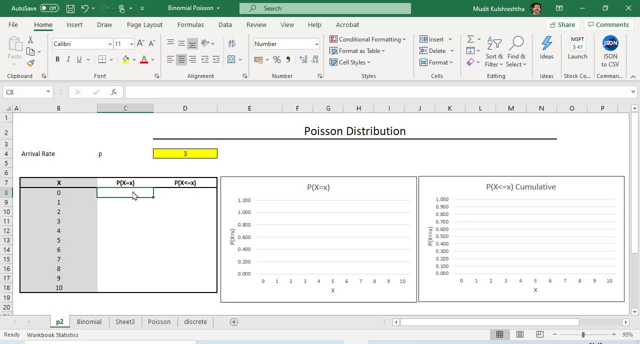 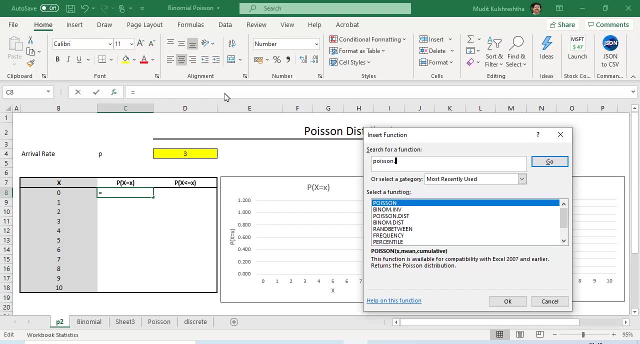 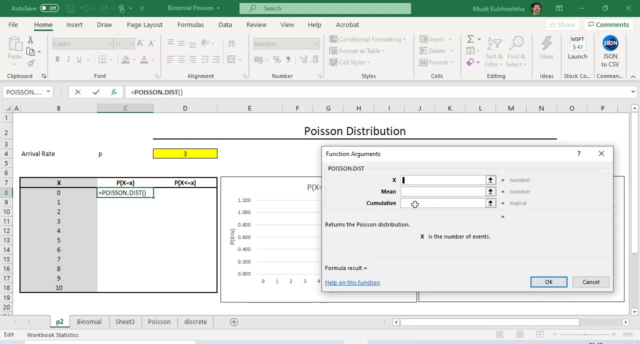 so Poisson distribution. go to the formula. wizard the formula for that is poissondist, so press go, and this is the formula that we are going to use. it's asking: where is the x value. so my x value is this. my mean value, arrival rate- is basically this: 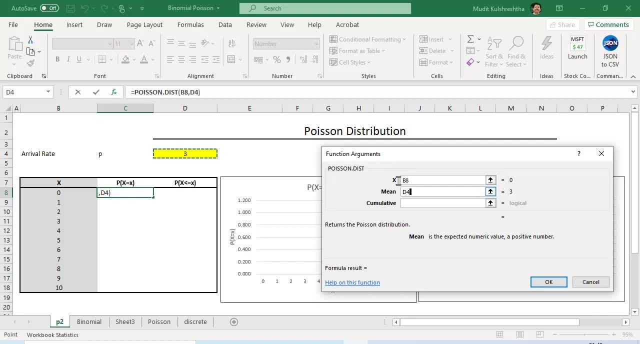 it's still labeled as p. we are going to change that to lambda, so dollar here and a dollar here as well, and cumulative. this will be false because we want to use the probability mask function, which means, for a specific value of a random variable, let's press ok and this is the probability. 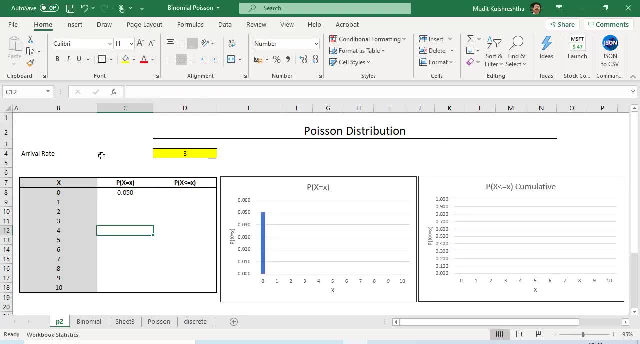 so let's name this lambda, or sometimes this is called as mu, and now I can just drag this. just make sure that the formula cells are getting picked right. yes, they are. we do that. and now to compute the cumulative value, I just need to copy the same formula. 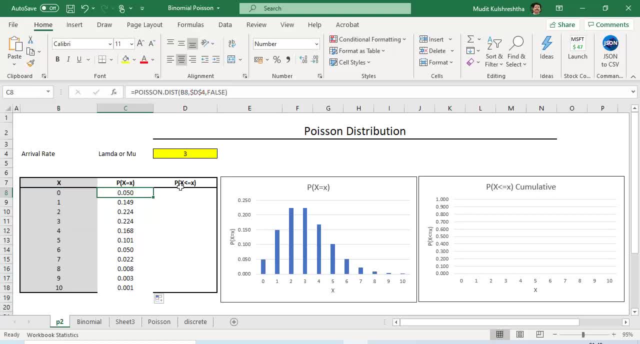 copy it in a adjacent cell and instead of false, we make it true, and that's it. I can complete the border here and now we have got all the tables and now you can quickly change this, so you will find that the graph will also change. now, remember that x can take values which are greater than 10. 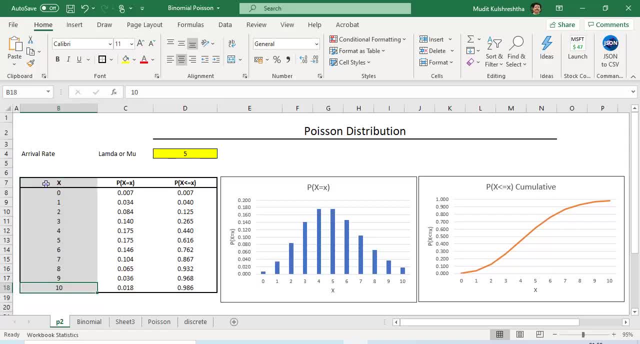 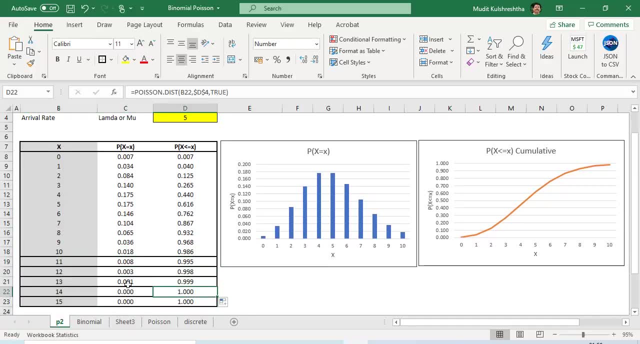 for poisson. so in that particular case, the only thing is that you can drag this down also for higher values, so that is the only thing that you will need. let me copy this formatting. of course, the graph still shows 10, so you can regenerate this graph. 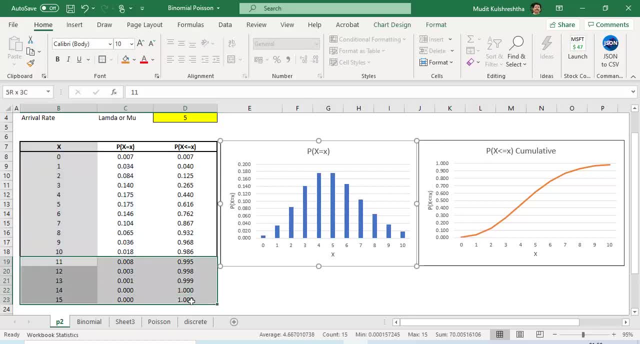 but I have just shown you how to extend this. in case random variable can take the values outside of 10- also in poisson, which is possible in binomial, the number of trials are finite. in poisson it is an infinite sequence. alright, so with that we have replicated both the binomial. 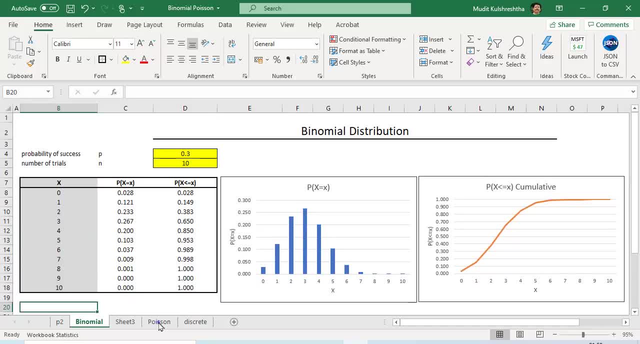 as well as poisson distribution modeling, and it could be pretty useful because this is like a ready calculator where you can just plug in these values and you can study these probabilities. so for example, suppose in binomial distribution you want to find out what is the probability where. 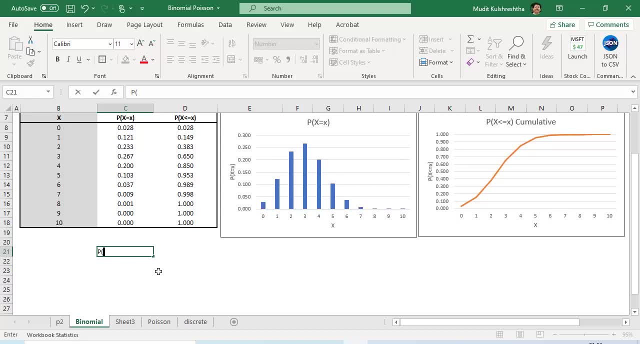 x is exactly equal to 3, we know that this probability is 0.267 or 26.7%, so these numbers can also be expressed in percentage terms and if we want to find out cumulative probabilities where x can take the value of 0.267, 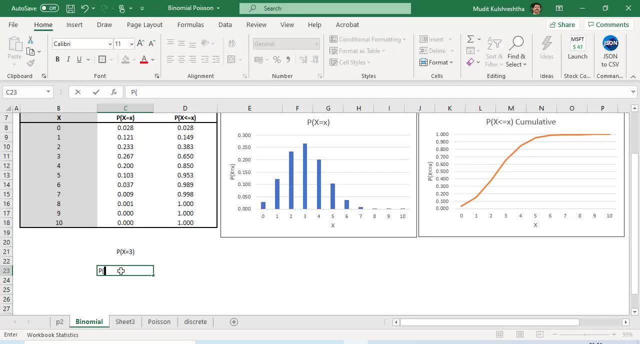 or 3, which means x is less than or equal to 3, then this probability will be found in the cumulative thing and this will be equal to 0.650 or 65%. so with that we have concluded how to compute the probabilities for discrete statistical distribution. 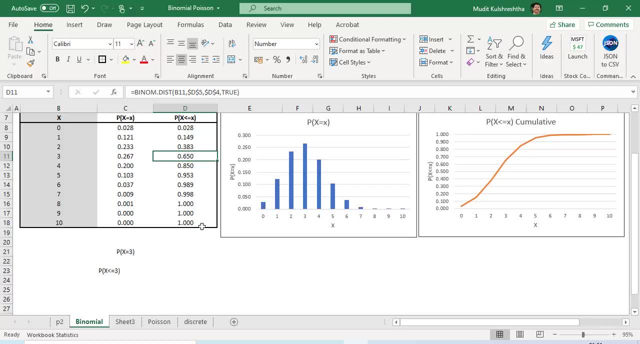 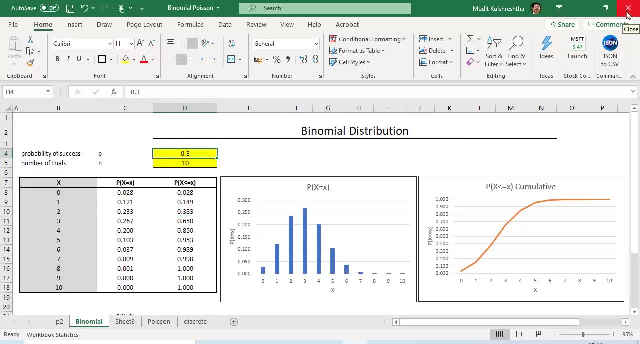 binomial and poisson. thank you for watching. if you like our videos, please do not forget to subscribe. thank you you. 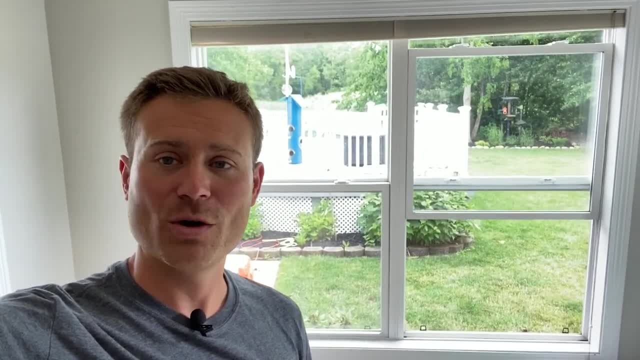 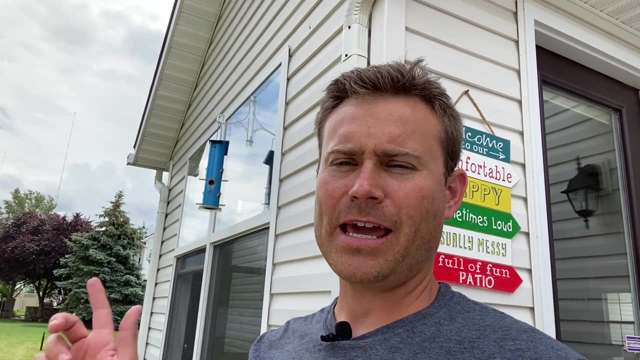 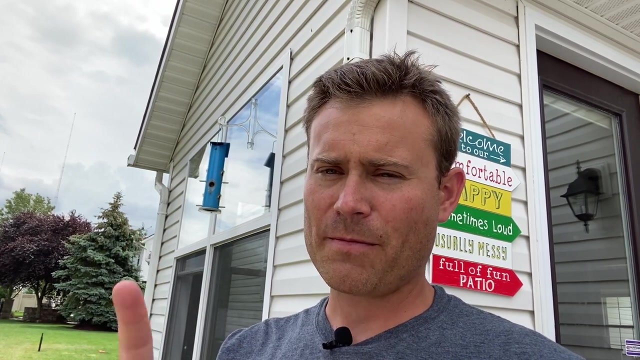 Hey, it's Scott from Bird Watching HQ, and today I'm going to talk to you about window bird feeders. All right, first, attaching a bird feeder to your window is just honestly, it's a ton of fun. but there is one very frustrating problem that can happen with your window bird feeder if you're not careful.